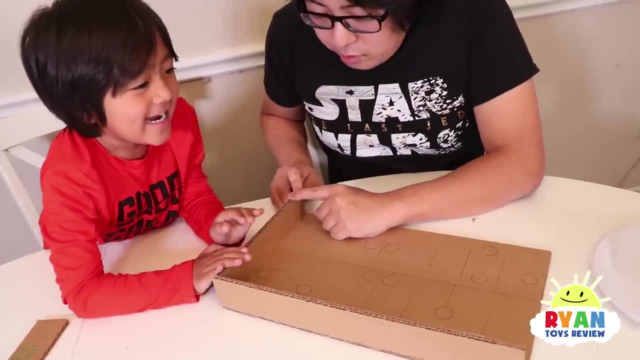 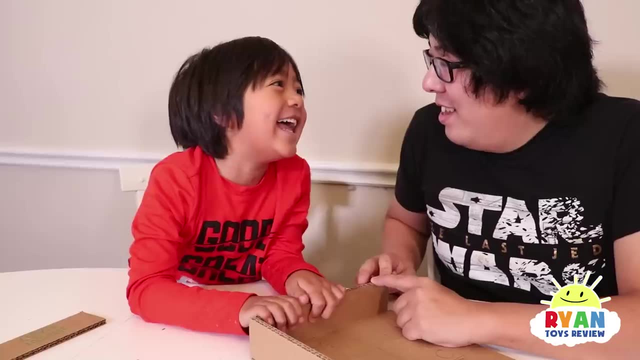 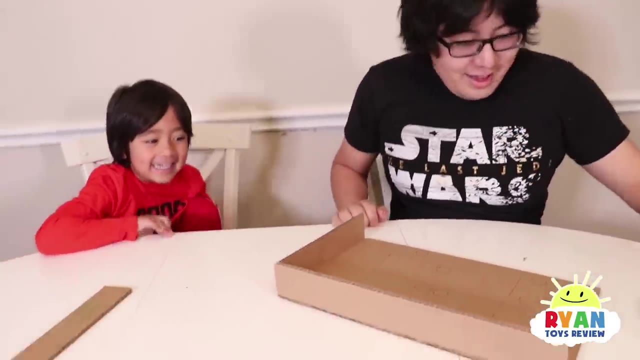 down ten, nine. oh, you're counting down seven, six, A million minutes. What One? What That's it? Are you sure that was 10 seconds? Let's see. Oh, yeah, you're right. Yay, it worked. Now we're going to do the other two sides. 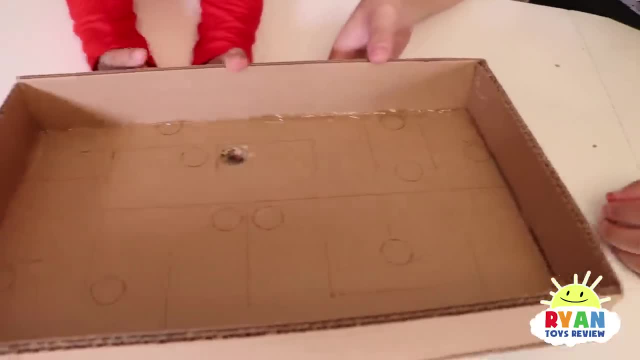 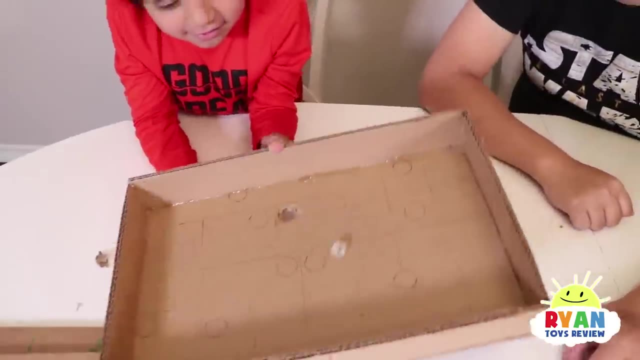 Now, Daddy glued all the sides and then we made a hole, so let's test it out, See if it goes through. Try to go inside that hole, Okay. Ah, it's so fast. Whoa, Holy, Whoa. 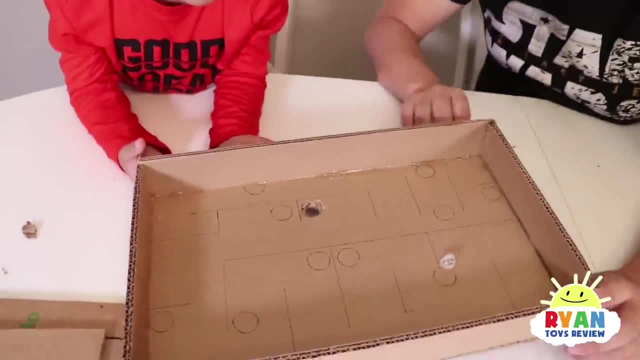 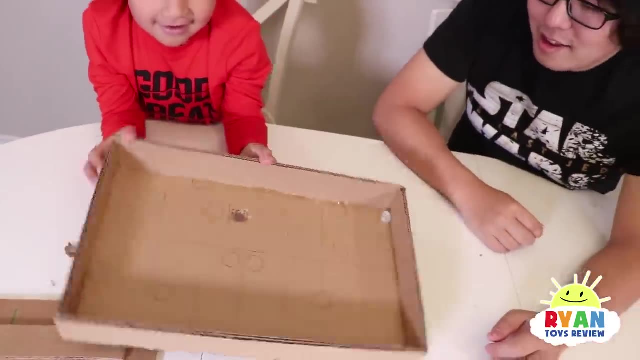 Whoa, It's stuck. Oh, it got glue. It's probably the hot glue. Ah, Sticky, Try to go slow. You want to go inside the hole Like off? Yay, Oh, whoa, Ah, I need to make the hole bigger. 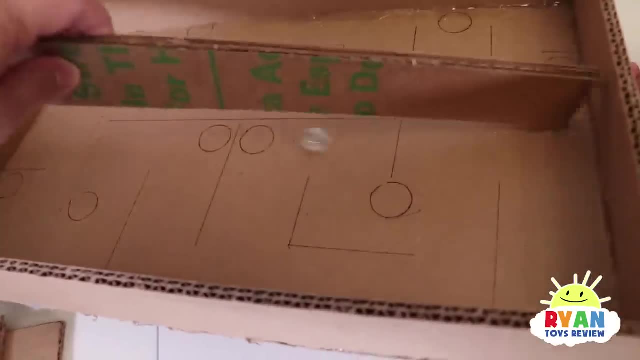 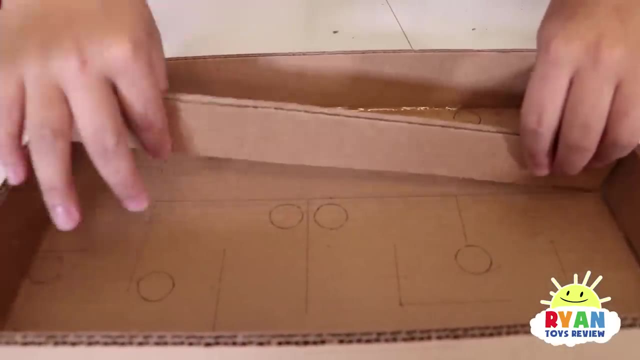 Yeah, so we got to make the hole bigger. Next, what we're going to do is cut and then paste it onto this little line here. Let's see It needs to be like around this one. This is where I cut. 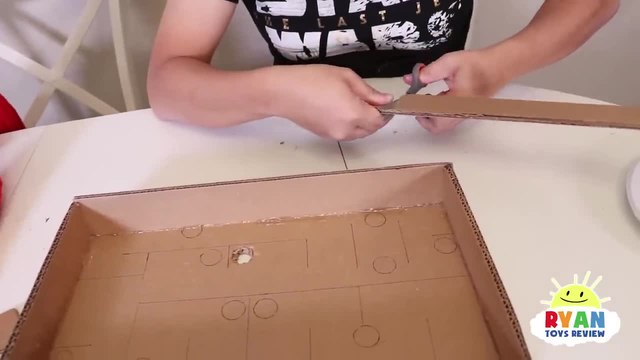 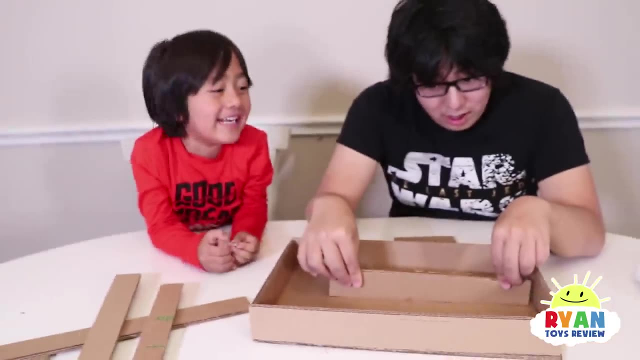 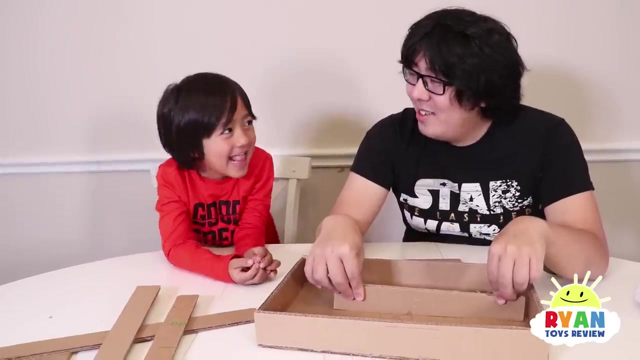 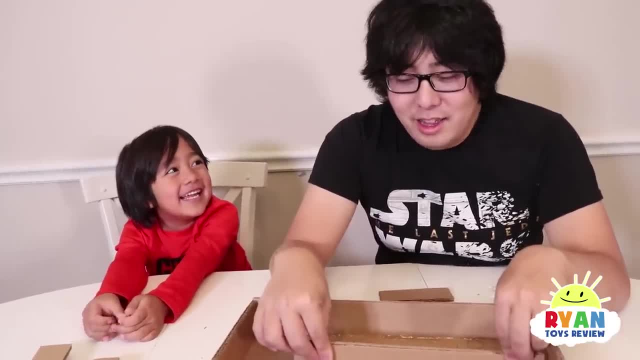 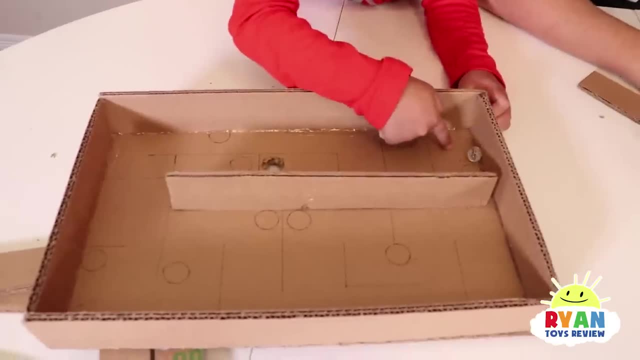 One, two, blah, blah, blah, 98,, 99,, 100.. Woo hoo, See, Whoa. I'm going to test it out. I'm going to disc it From this corner to that corner, OK. 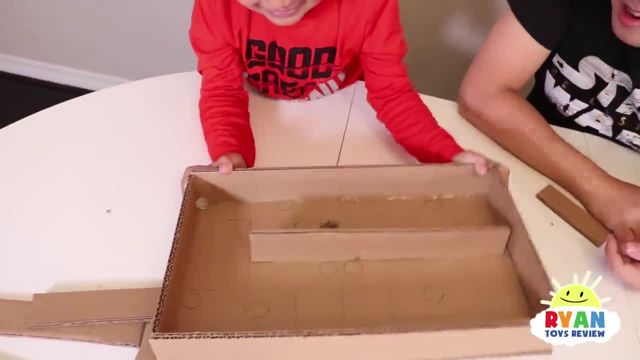 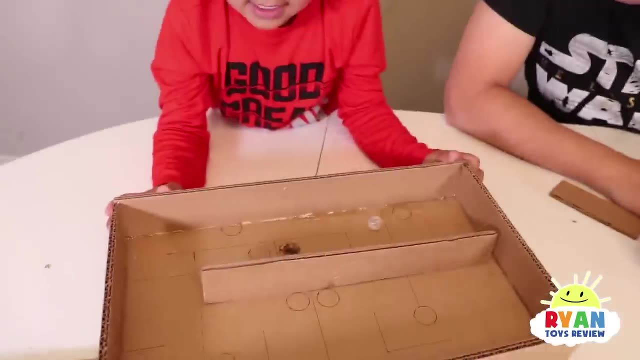 Don't fall in the hole, Don't fall into that one hole. Whoa, He tilted so much. Oh, Oh easy. Oh really, You made it OK. so now we're going to finish pasting all the sides. 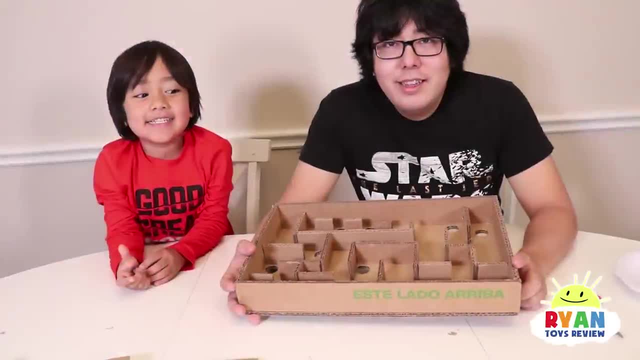 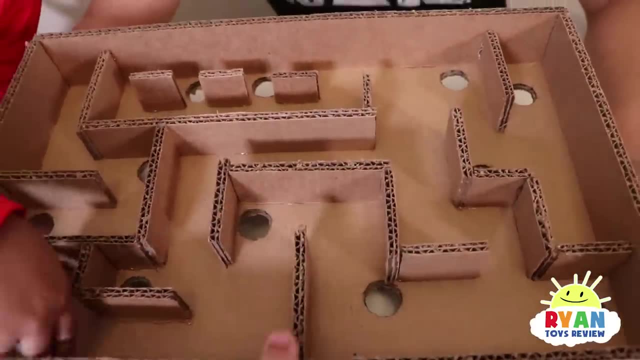 And then we're also going to finish cutting the holes out. So it's done. Yay, looking cool, Looks like a real maze now. So we did all the holes and glued in all the pieces. So now we have to Mm. 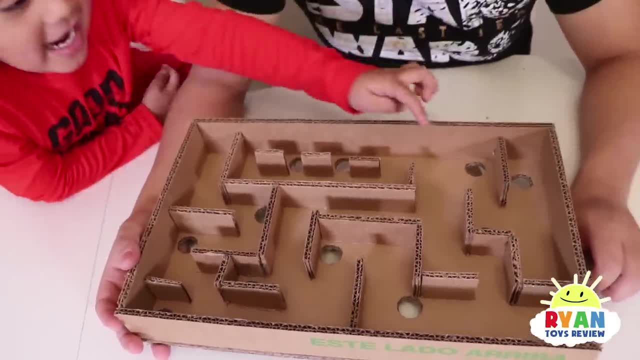 Pick: where do you start and where do you end? Yeah, where do you want to start, Ryan? I want to start right here. Start right there, Maybe like right here. Oh yeah, That's where you start, Yeah, Start. 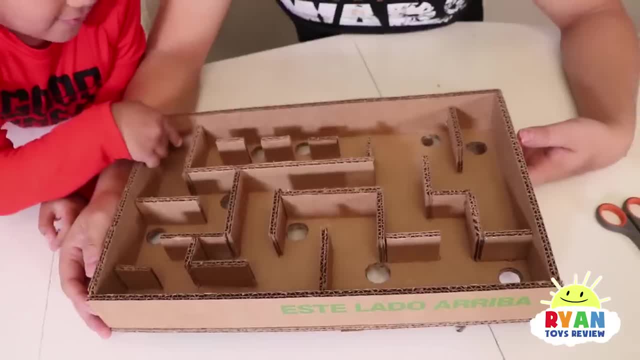 OK, And then where do you end? In this corner, In this corner. OK, Daddy, you try, Can you do it? Oh, Oh, Oh Oh. Of course not. I didn't even see that, Oh no. 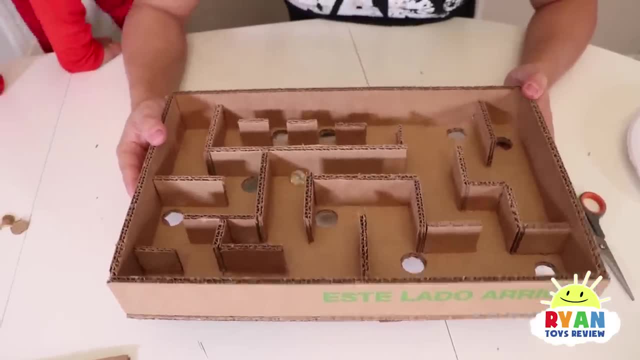 I can do this. I can do this. Whoa, Whoa, Whoa, Whoa, Whoa, Whoa, Whoa. I can do it better than Daddy. Give me more points, because I'm going to go fast. 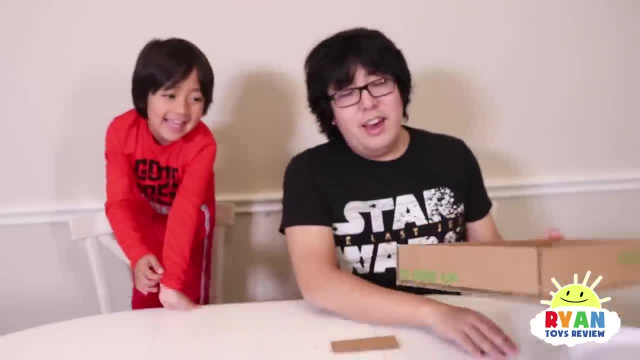 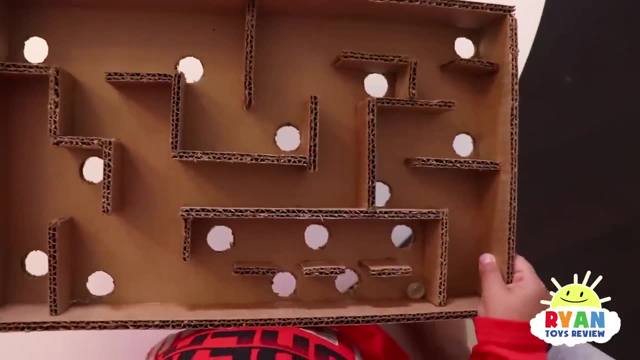 Oh, that's hard, right there. Oh Oh, Oh, There's a hole. Oh, I didn't see it. Oh, Ryan, it's hard. Maybe we should do a different start and finish: Whoa, Whoa. 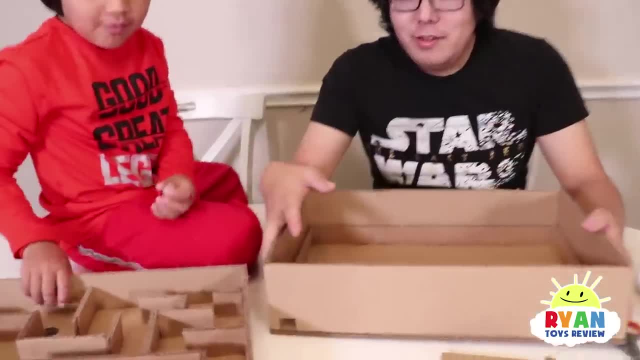 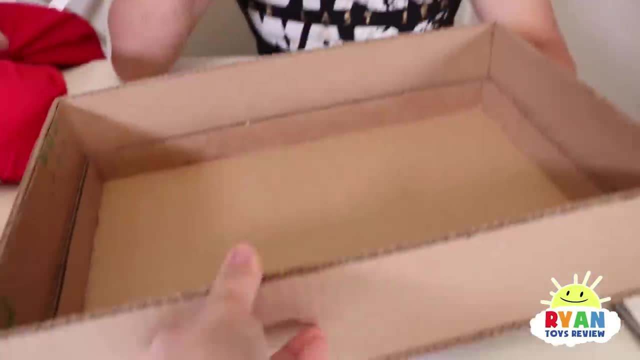 Wow, We also made a bottom. Should we bring the spools? It doesn't go all over the place. Yeah, So the bottom. it just looks like this: We just glued four piece on the outside, Four, And then four piece on the inside. 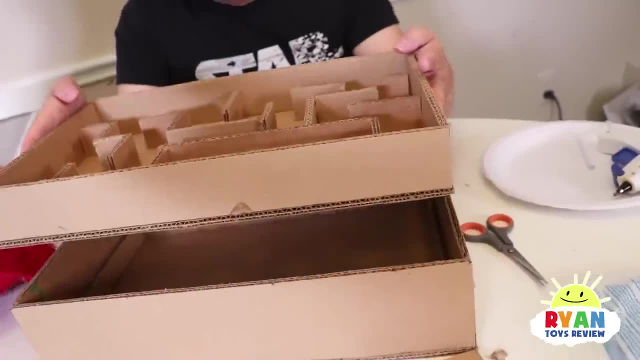 And then we also cut a little bit and made a little hole here so the marble can come out. Let's test it out. So I'll hold it like this: Can you drop the marble through the hole? See, it goes in there. 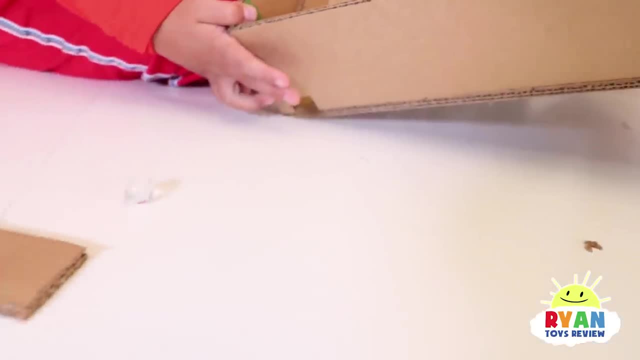 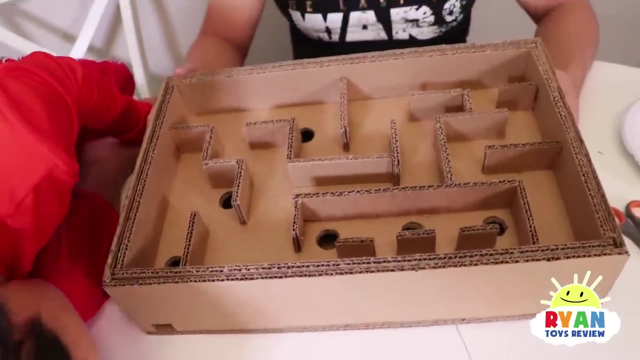 And then you roll it out the hole. Whee, Now let's put it together. This should fit. Oh Whee, Awesome, But nice. Now I wrote start and finish on a piece of tape. Yeah, So all we did was we just got tape. 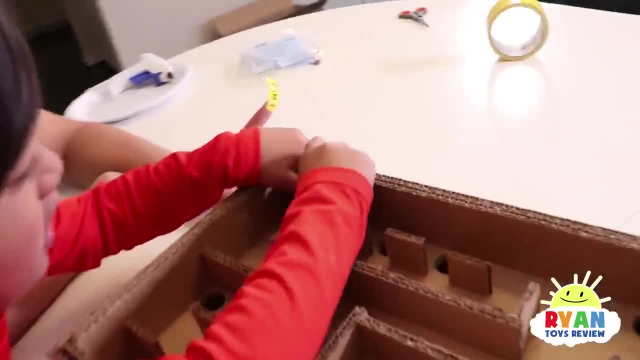 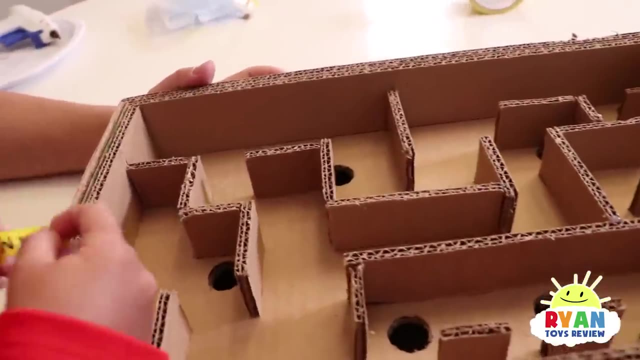 wrote down start and finish. Ryan is taping in the start. There we go. So that's where we start. Where do we finish? We're going to finish right here. right, Finish Like this. Yeah, That looks good. 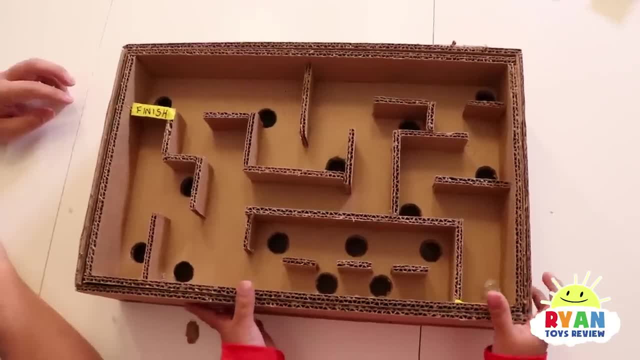 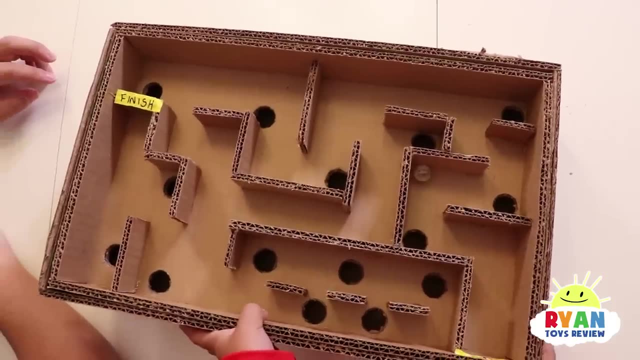 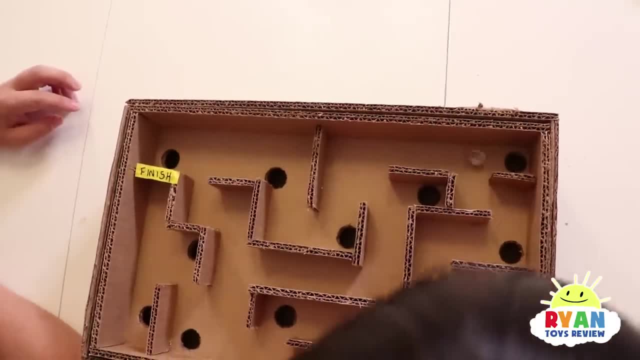 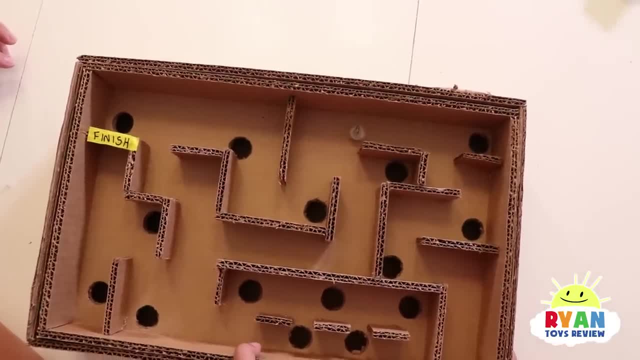 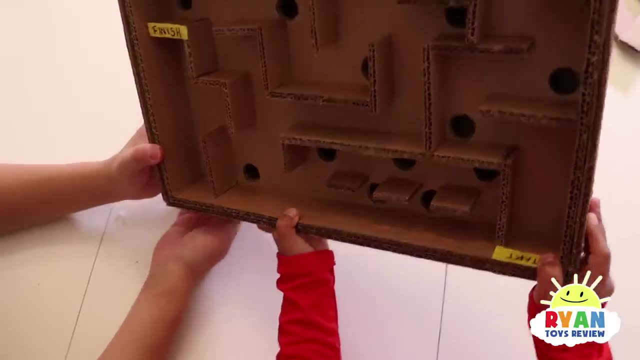 Whoa, Whoa, Whoa, Whoa, Whoa, Whoa. You're doing really carefully. Nice, Oh, Nice, Ooh, Oh, Oh, Ah, Nice, It's OK, we have a hold or we can get out. 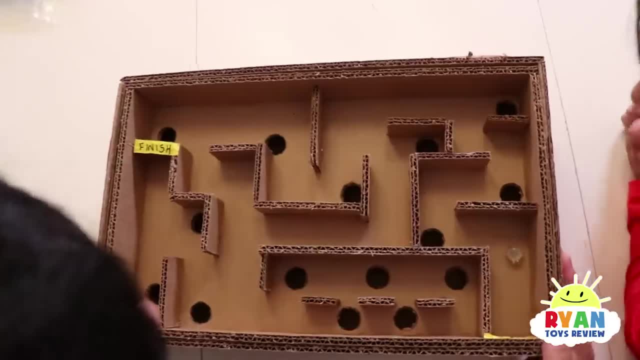 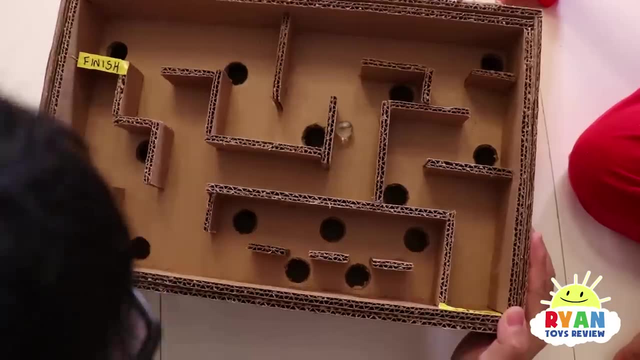 Our daddy's going to try. Yeah, I'm going to try. OK, daddy, I've finished this before, Did you? Well, only one time You do it. Uh, that was close. Yeah, Yeah, Did you find a shortcut? 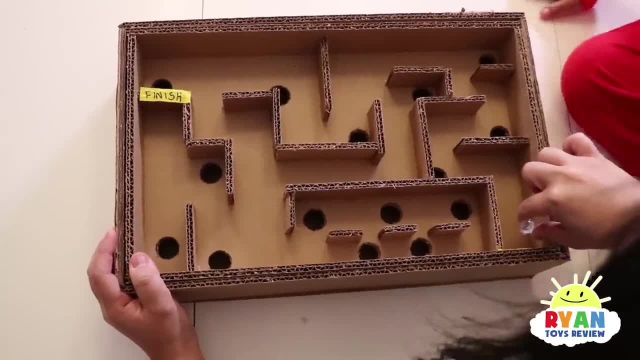 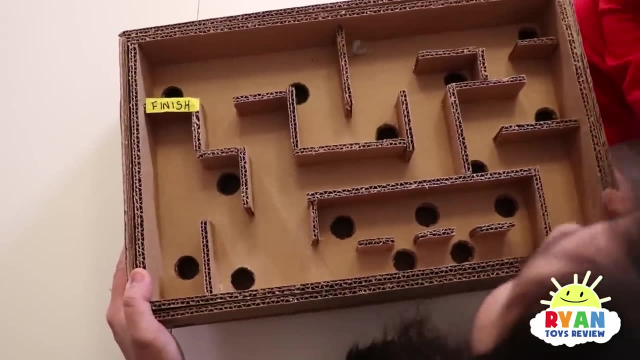 Whoa, I want to try. Okay, mommy's turn. Let's see if I can do this. Follow daddy, because there's no hole in it. That way it looks cool. Let's see. Can mommy do this? Can mommy do this? 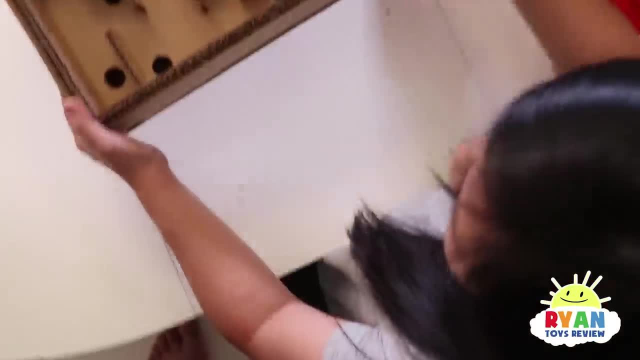 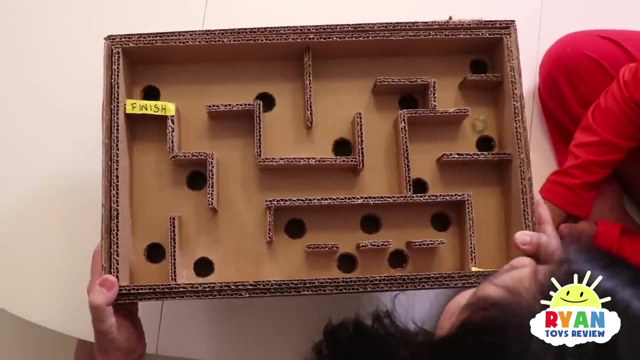 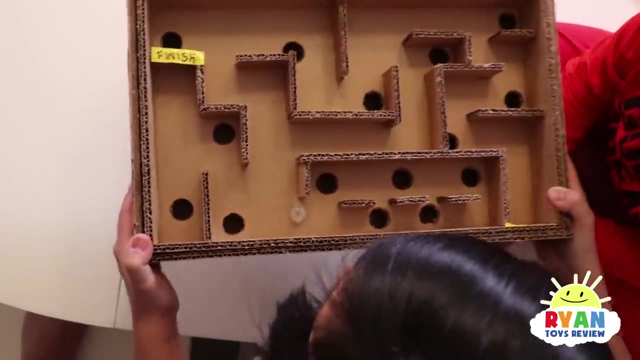 Mommy cannot do this Ready. I want to try again One more time. This is so much fun Following my task. No, no, no, I did it. Good, good, good, Wow, it's always so much fun. 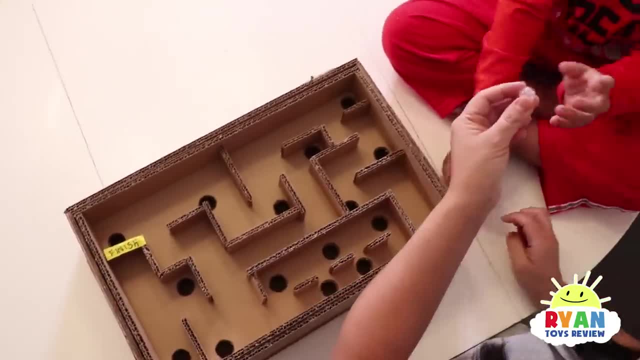 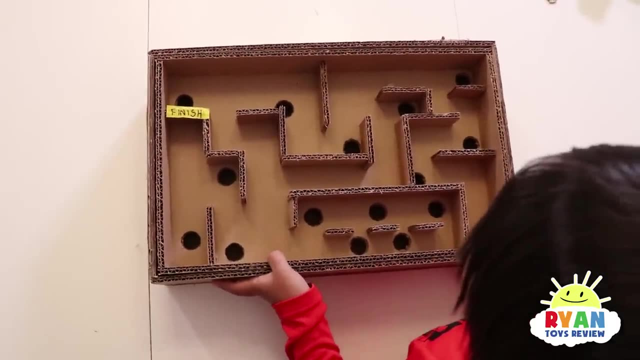 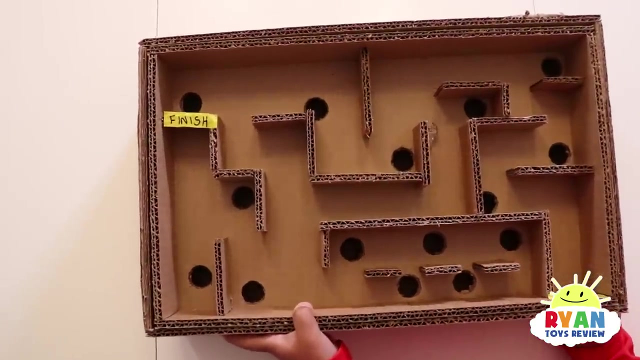 when you create your own toy right? You want to try My turn? I'm going to try. Good, good, You're still doing good, You're doing great. Nice, He's super careful. Good, good, good. 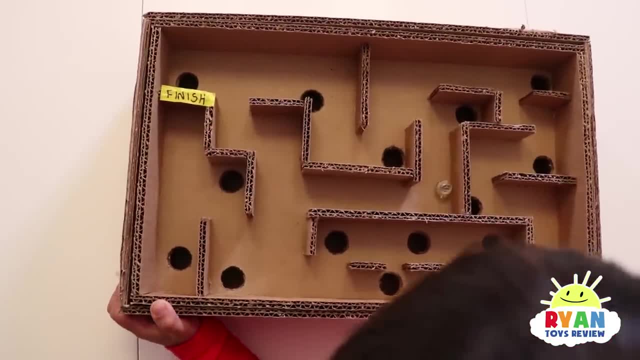 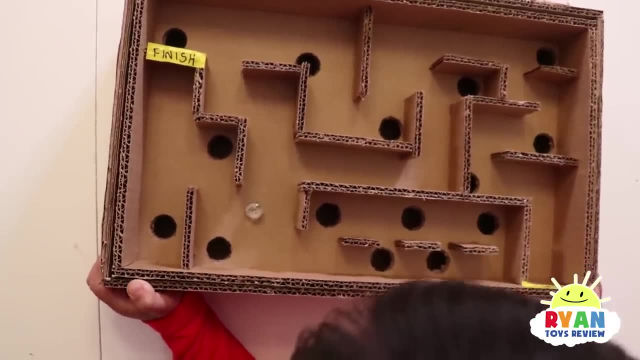 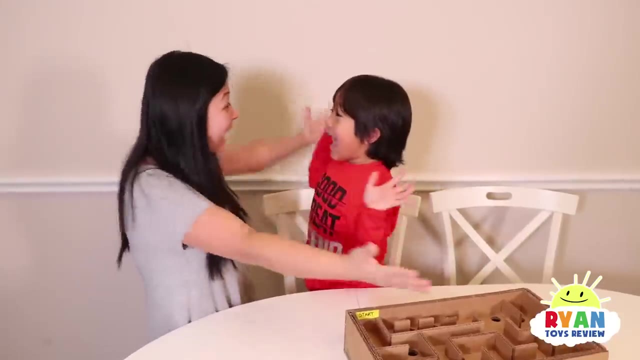 Go left, Left, go left. Oh, that worked. Oh, that's the difficult part, Ryan, Slowly, Almost, Almost there, You did it, Ryan, and daddy did it, but mommy haven't done it yet. I want to try again. I need to beat this. 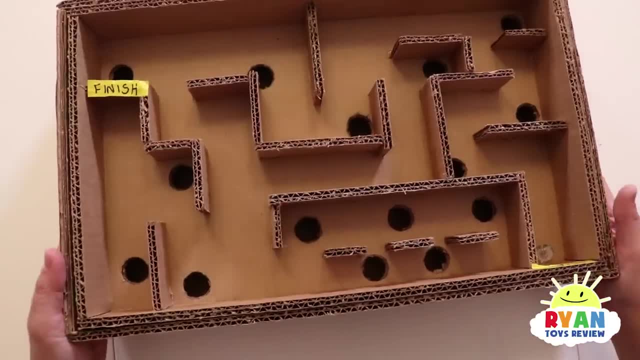 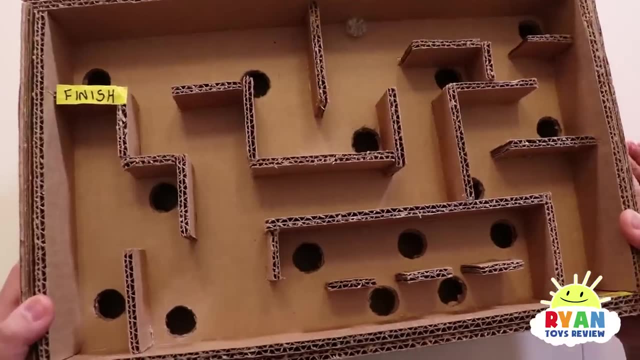 Even Ryan can do it. All right, let's go. I need to be able to do this, Come on, Come on. You can't see it. If you can't see on the hole, I'll tell you There's a hole there. 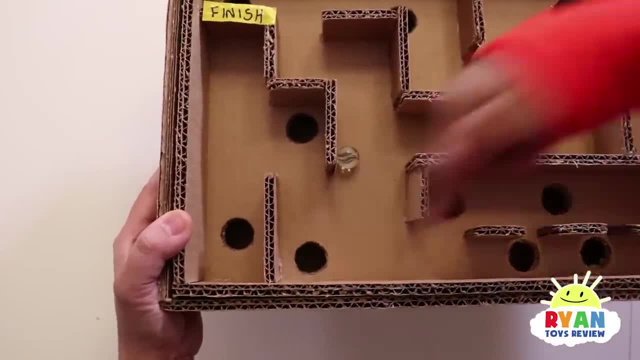 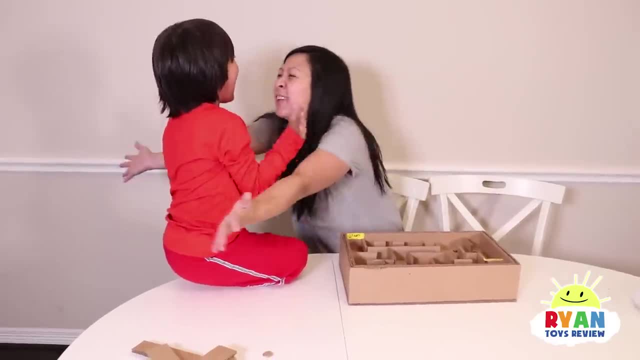 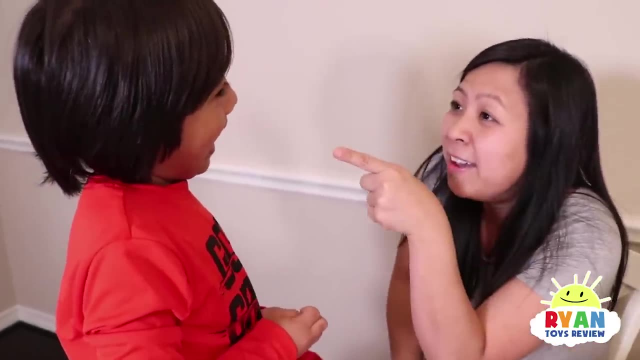 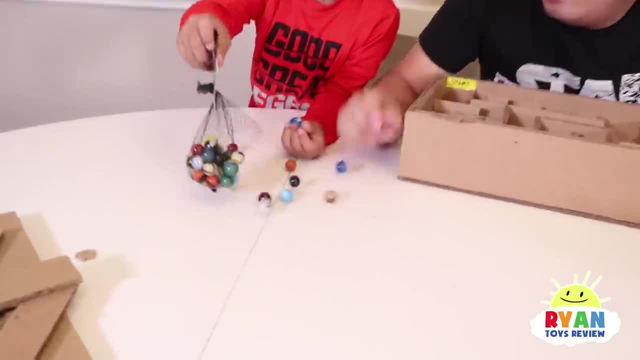 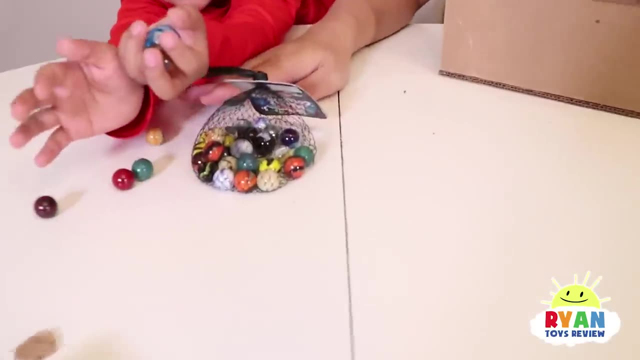 Are you ready? Yes, Okay, We have a whole lot of different models. Wow, Wow, Wow, Wow, Wow, Wow, Wow. And different colors and different sizes. Yeah, so there's so many different marbles. We're going to do a marble challenge. 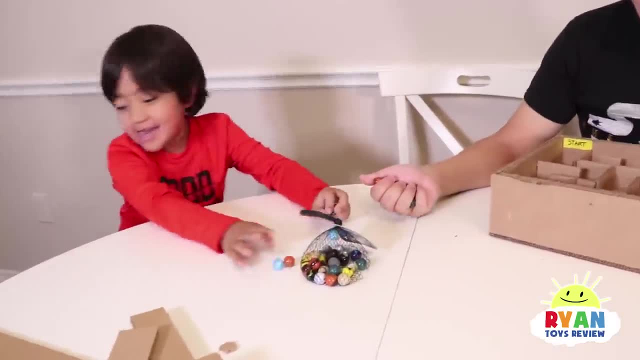 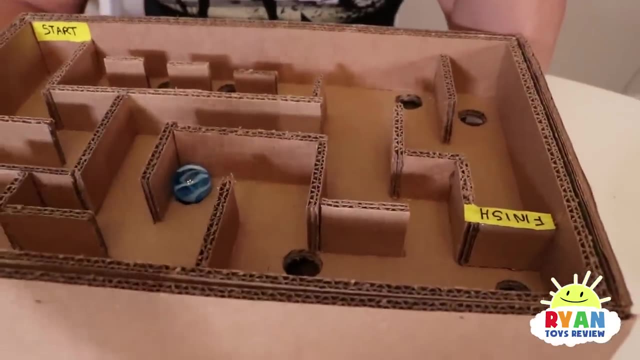 and put more than one in there to see There's way more than one, Yeah, and some of the marbles. we got two marbles in here that are giant size. It won't even fall in the hole, Will it? Yeah? 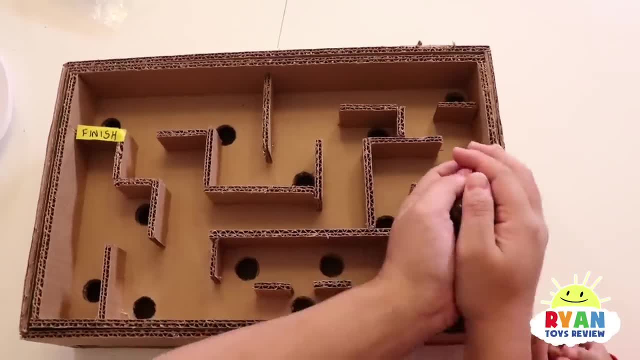 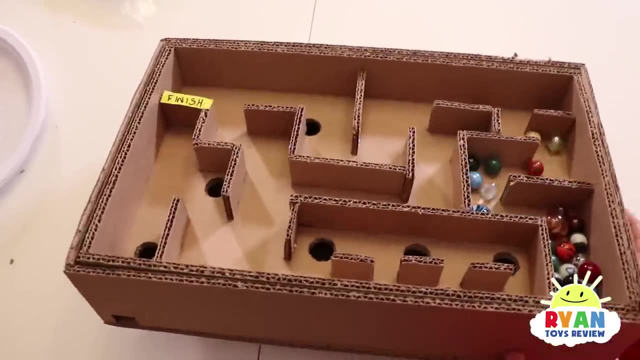 See, Oh, Daddy's going to put a whole bunch in here for Ryan. Whoa, All right, See how many he can guide you. All right, Let's see how many can he guide to the finish line. Let's see how many he's going to make it hang. 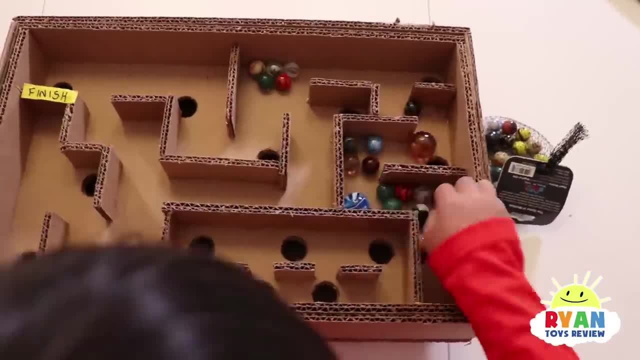 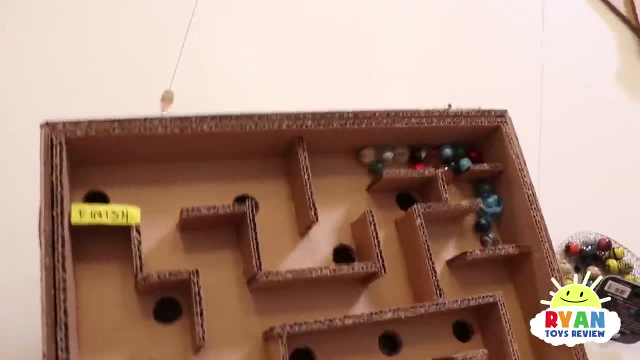 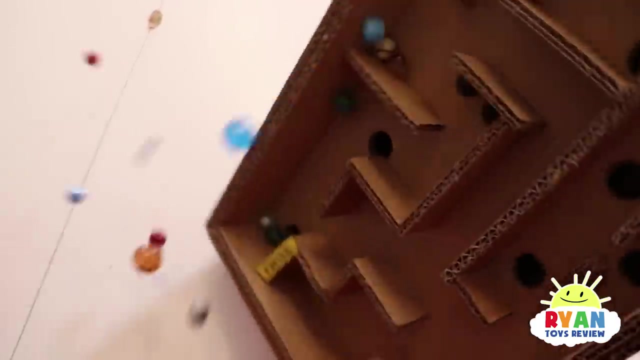 I think it's stuck there. It's stuck so many. There you go, Shoot, I thought these were hanging. Yeah, it's stuck. There you go. let's see How many can he guide to the finish line. We're going to try again, with a little bit less. 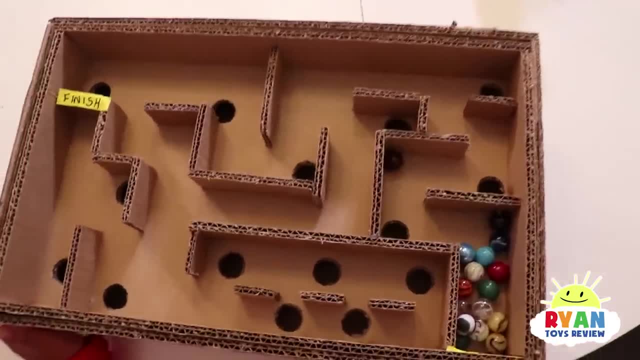 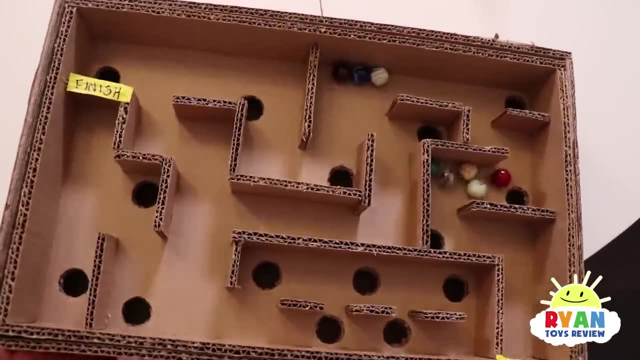 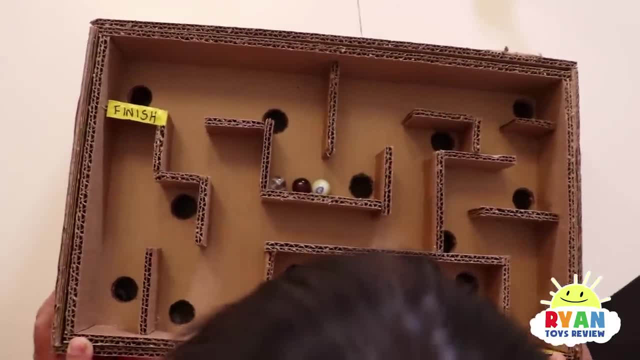 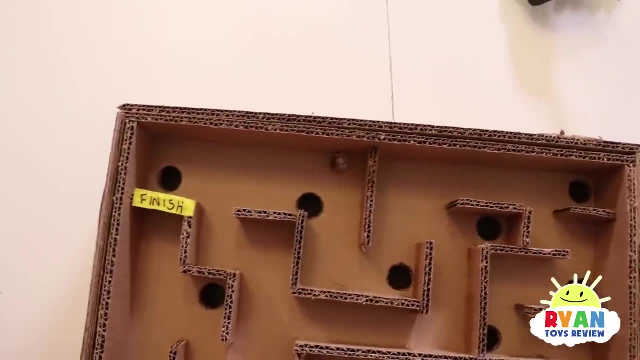 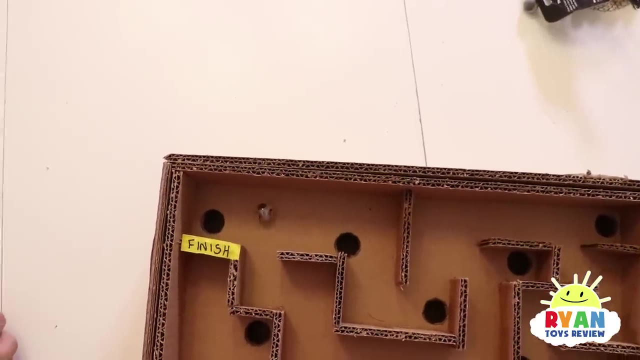 Wait, wait. This way, You only have three left. Oh no, I'm not going to win. Oh my, oh my, I'm scared. that's why it's not falling into the water. You're doing great, There you go. 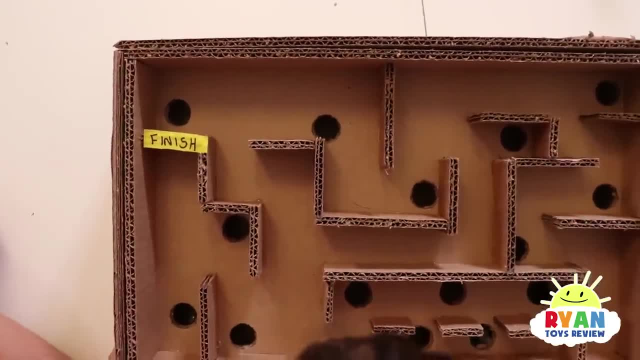 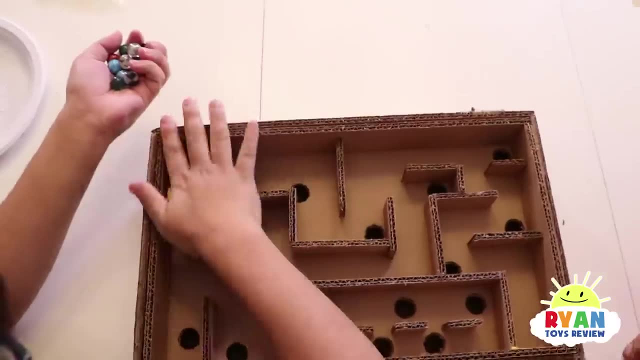 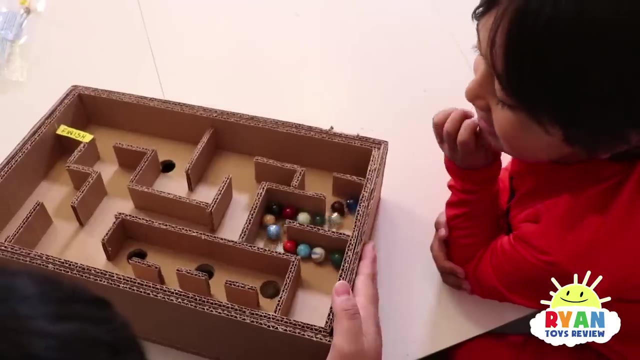 Go over, go down. Oh, wrong way, wrong way, Wrong way. dude, Daddy want to try? Yeah, sure. And then, mommy, Is it a lot harder with more? Ryan, Huh, Is it a lot harder with more. 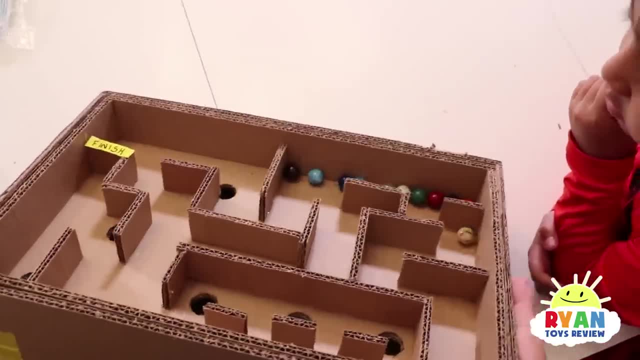 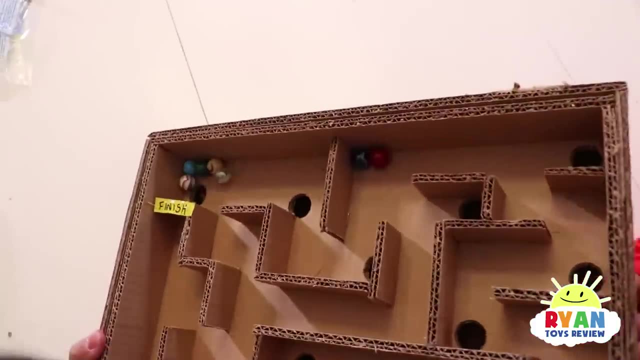 Yeah, It's hard to control with a lot of water. Yeah, that's why it's the ultimate challenge. But you don't have a lot of chances if you don't have a lot. Oh, daddy's pretty close, Oh my. 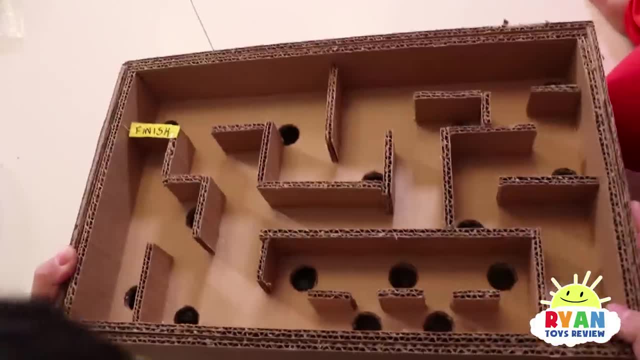 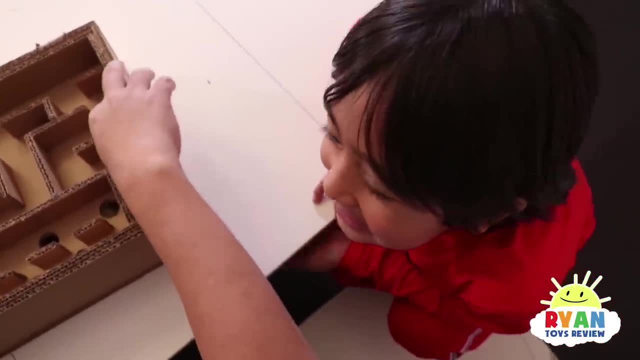 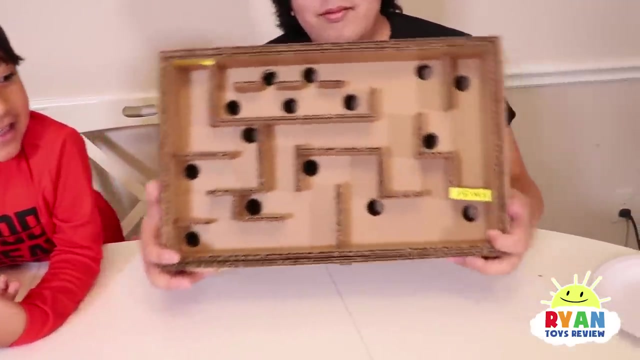 Ah no, Oh no, Oh one. This is harder. I was better because I was staying longer. That's true. Bye. thank you for watching our video. Bye, and please let us know what other things we should try to make.